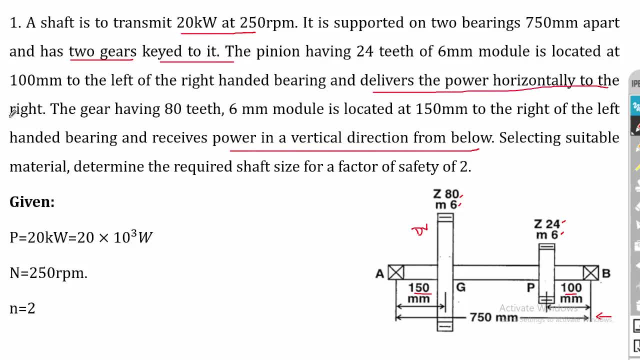 And the pinion delivers the power horizontally to the right. So the pinion delivers the power, which means it is the driving gear. So this is driving and this is driven. Select suitable material, Determine the required shaft size For a factor of safety of 2. So in the problem two gears are there. So the pinion is a driving. 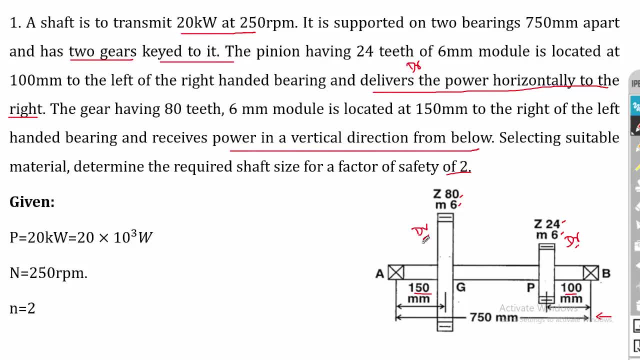 gear and the gear is a driven one. So the pinion delivers power horizontally to the right. So another gear is fixed in the horizontal direction at the right side. So when you view from the left hand side, then this is your pinion. There is another gear- mating gear- is on the right side, So this is our shaft. So for this shaft we have to calculate the diameter. So this pinion delivers the power to another gear horizontally to the right. 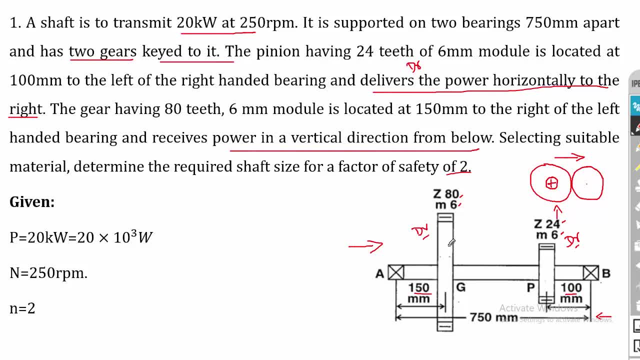 Then this gear receives power vertically from below. So this is your gear G, So you can name it as G And another one as P. So this is your gear G And it is fixed in the shaft, So it receives power from another gear vertically below it. 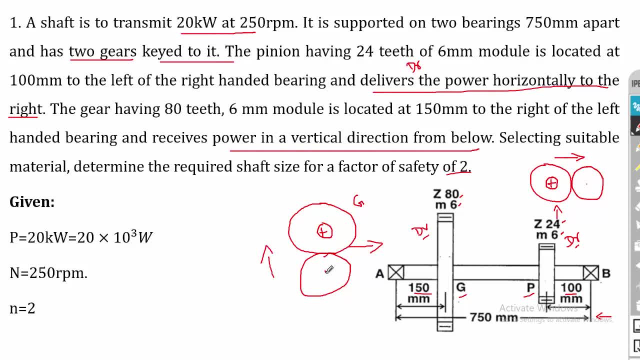 So this receives the power vertically below it. So now it's a driven gear and here it's a driving gear. But one thing is not given, that is the direction of rotation. So here the direction of rotation of the shaft is not given. So if in the problem, if it is not given, then we can assume any one of the direction. So in this problem, what I am going to do is I am going to assume the shaft is rotating in counterclockwise direction. 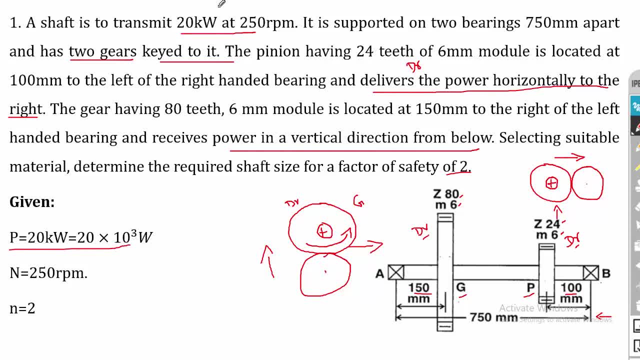 Ok, So first we will write the given data. The power is at 20 kilowatt, So 20 into 10 power, 3. And speed is 250 rpm, Then factor of safety is equal to 2.. Since the material is not given, we have to select the. 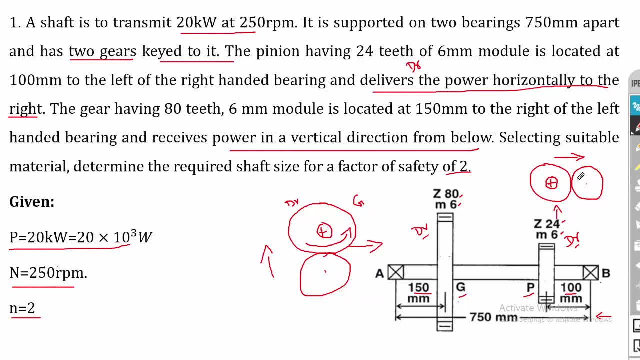 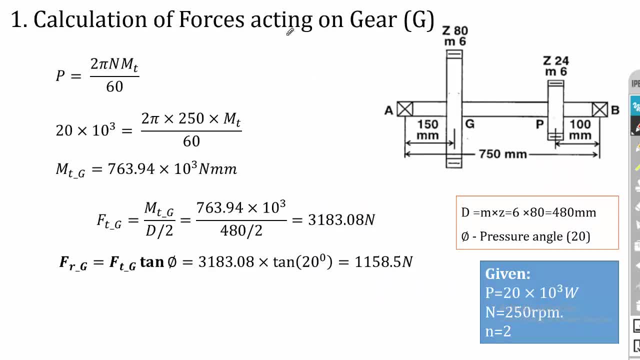 suitable material. Ok, So here these two drawings are the left side view, Be clear about it. Ok, So the first step is calculation of forces acting on gear. Consider the gear G. Ok, Fine, So first we will calculate the FT and FR before going to the force drawing. We know that P is equal to 2 pi NT divided by 60.. In the problem, P is common for both the gears. So that is. 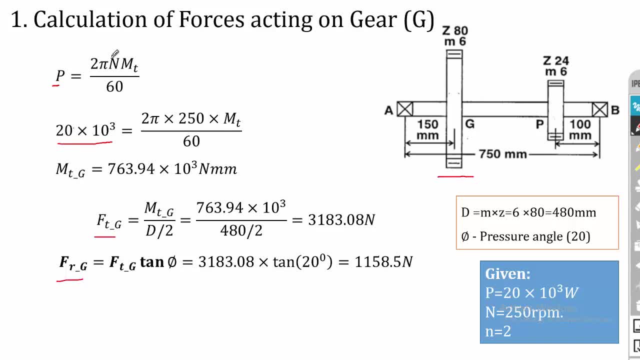 is 20 kilo newton, you can put 20 into 10 power 3, then 2 pi n is given. it is 250 rpm. so 250 into empty divided by 60, so we will get empty in newton meter. convert it into newton mm, you will get empty. 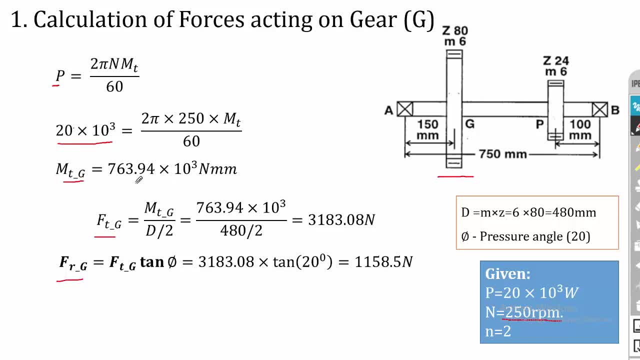 g that is empty, acting on gear is equal to 763.94 into 10 power, 3 newton mm. further, we know that ftg is equal to. i have already given you the equations: ftg is equal to mtg divided by d by 2. 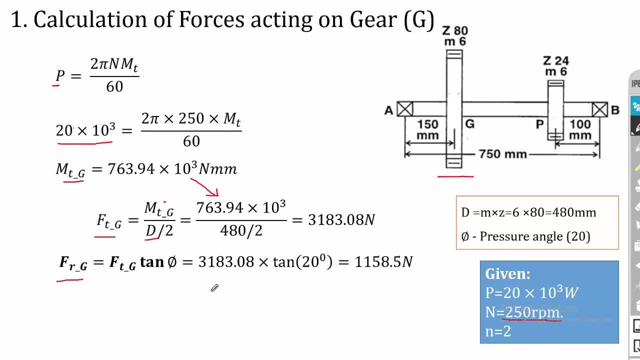 so mtg i have calculated. d is the diameter of the gear. so actually in the problem the diameter is not directly given but the module and the number of teeth is given. so for the gear g the module is 6 and the number of teeth is 80. so m into z is 480 mm. that is the pitch circle diameter. 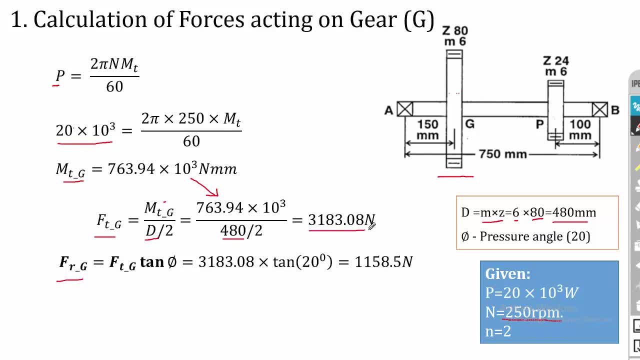 of this gear. so we can substitute that. further. we can calculate: ft is equal to 3183.08 newton. further, frg is equal to ftg, that is ft tan phi. in the case of g it is ftg tan phi. okay, so phi is pressure. 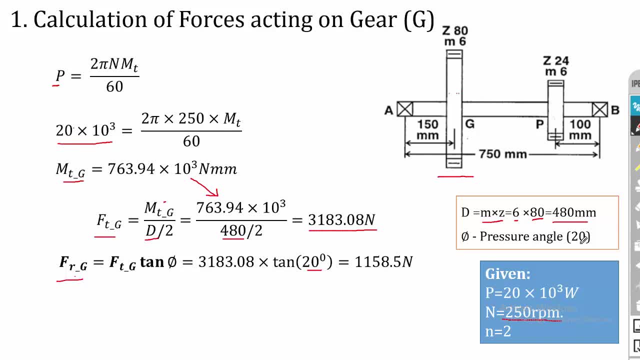 angle in the problem. the pressure angle is not given, so you can either take 14.5 or 20, okay, so here i have considered 20 degree. so the frg is 1158.5 newton. so now i have calculated the tangential force acting on gear and the radial force acting on the gear. so now i have to draw. 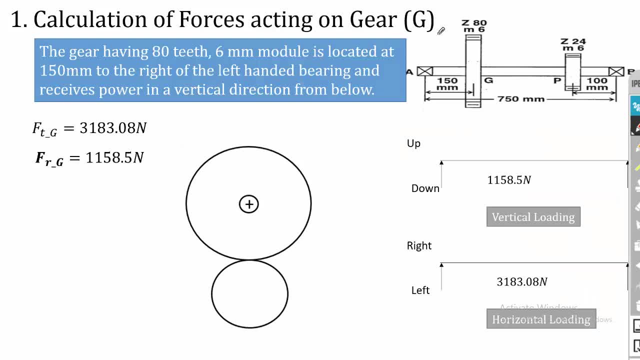 the force diagram. okay, so this is the given drawing and in the problem it is clearly stated that the gear having 80 teeth, 6 mm module, that is, gear g, is located at a distance- okay, to the right, of the left handed bearing and receives power in a vertical direction from below. 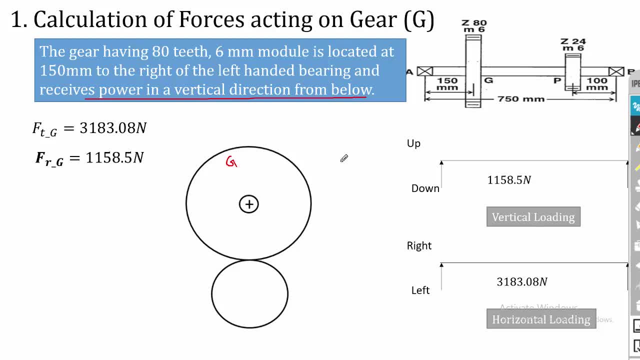 So this is the gear G, and it receives power in a vertical direction from below. So here this is the driving shaft, and here our gear is a driven one. And in the first step I have assumed that the shaft is rotating in counter clockwise direction. 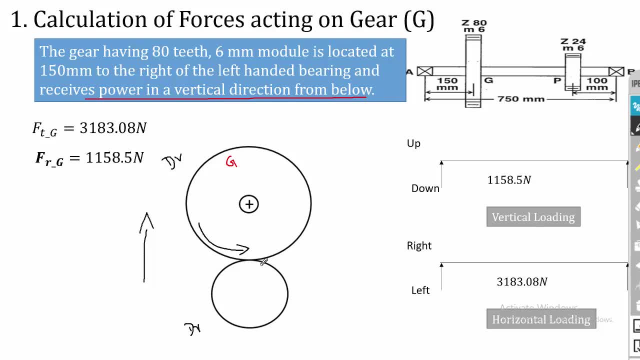 Remember that since it is vertical direction and it is below, I have drawn the mating gear in the bottom. So this is the left side view of this shaft And I have assumed that the shaft is rotating in counter clockwise direction. So if this gear rotates in counter clockwise direction, then the mating gear will rotate. 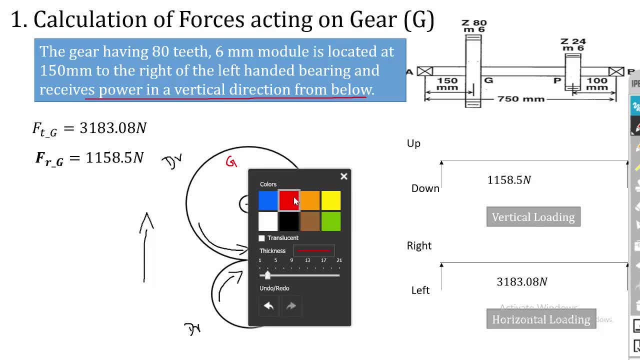 in clockwise direction. Ok, And as I told in the previous class, always the driving gear will deliver the power and the driving gear will apply a force on the driven gear. So here this is the driving gear and it is rotating like this. So if it rotates like this, then this will deliver a power of F in this direction. 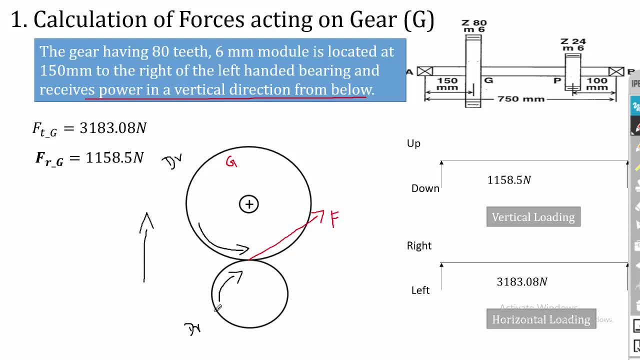 So be clear about it always: the driving gear will deliver the power. Ok, So the power will act. The force will act on the driven gear. So here in our problem, the driven gear is actually fixed in the shaft, so you can directly consider the force. 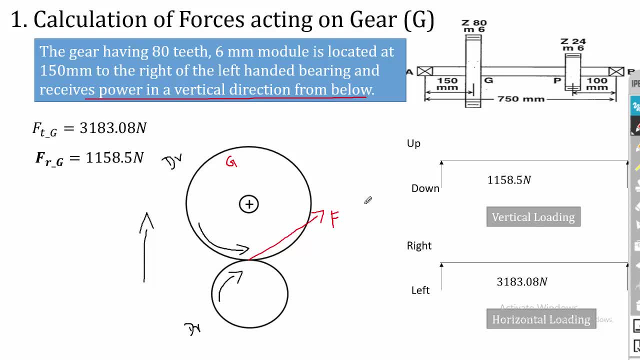 So since it is rotating in clockwise, the force will act in this direction, So further. we can split this into two components. One is the tangential one, Ft, and the another one radial force. Fr Ok, So Ft and Fr Ok. So these two components we have already calculated. 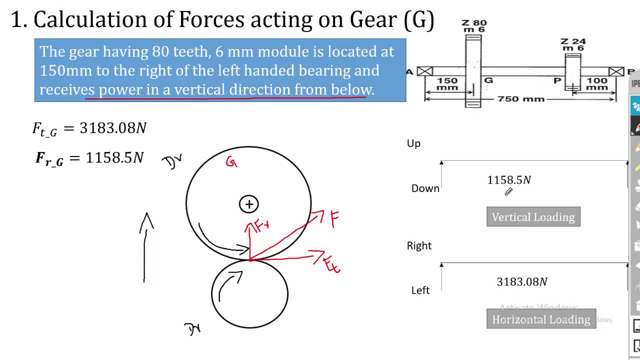 So by having this force diagram then we can move into the vertical loading and horizontal loading drawing. And remember that in vertical loading it is up and down and in the horizontal loading it is right and left. So the overall length and it is supported on two bearings so you can assume it as a simply 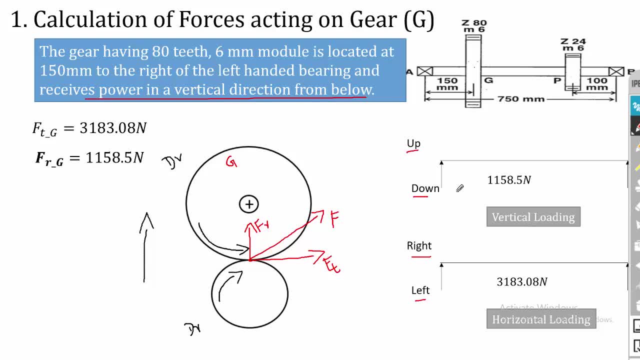 supported beam. Ok, Fine, So first consider the vertical loading. Ok, So in this arrangement the Fr is actually the vertical load and it is moving towards upward. Ok, So you can draw Fr, it is moving towards upward, Ok. And I have mentioned the magnitude, that is 1058.5 Newton. 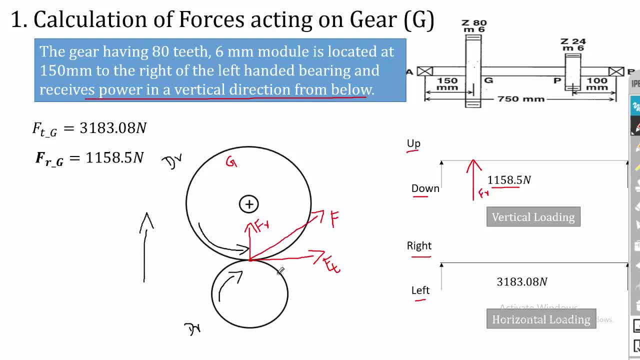 Then the horizontal loading. So Ft is the horizontal load and it is acting towards right. So from left to right it is acting. So it is acting towards right. Ok, So the magnitude is 3183.08 Newton. Ok, So this is for the gear. 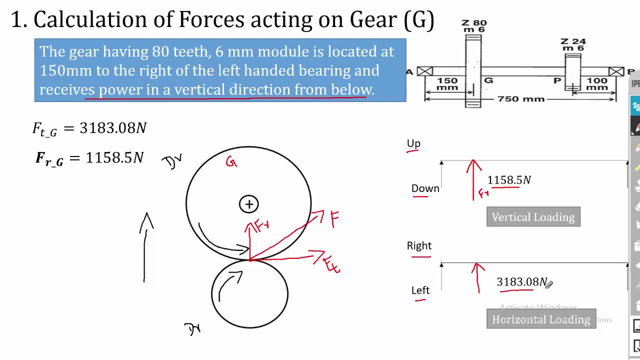 Remember that the gear is a driven one. The driving gear applies the force on the driven one. that is why we have not considered the reaction force. Ok, If the gear fixed in the shaft is a driving one, then we have to consider the reaction force. 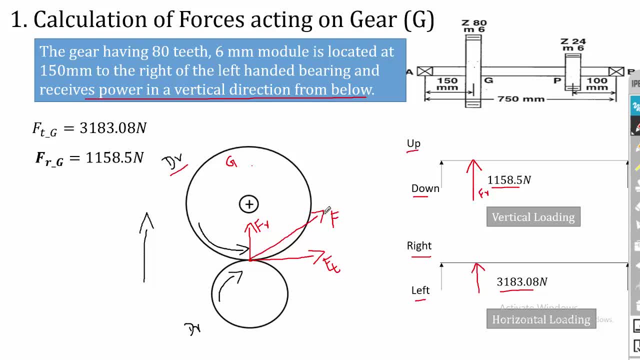 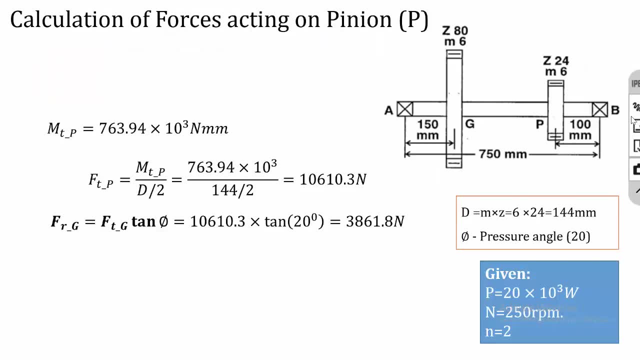 In this case it is a driven one, So you can directly take the forces. Ok, So this is for the gear G and the next one is for the pinion. that is the next gear, that is P. So we have to calculate the Ft and Fr at the initial stage and the torque we have. 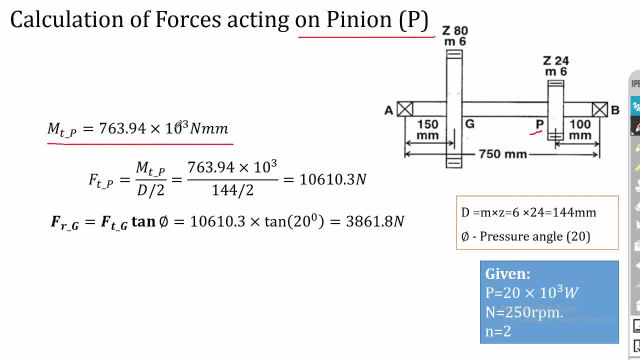 already calculated in the previous step, that is 763.94 into 10 power, 3 Newton mm. Further, the Ftp, that is the tangential force on P, is mtp divided by d by 2. So, like the gear, here also the diameter is not directly given, but the number of teeth. 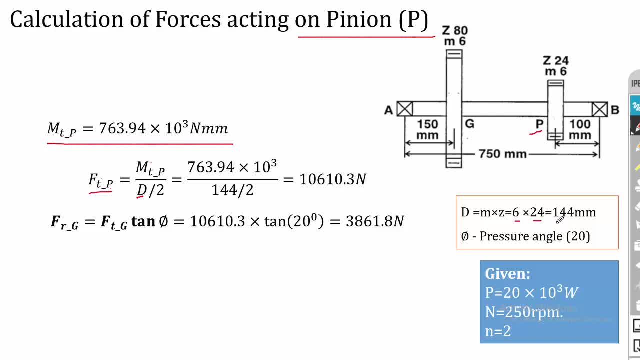 and the module is given. so by having this we can calculate the diameter of the pinion. so that is 144 mm. So now we can substitute the mt value and the diameter value and we can calculate the Ftp. This is the diameter of the pinion. 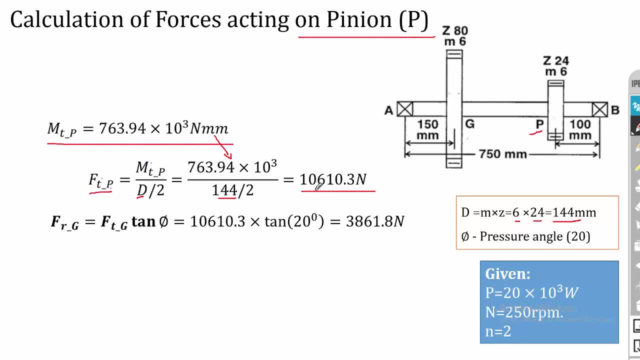 Ftp, that is tangential force acting on the pinion. that is 10610.3 Newton. So after calculating Ftp you can substitute in this equation this is actually Ftp. So Frp is equal to Ftp tan phi and I have assumed a pressure angle of 20 degree. so you 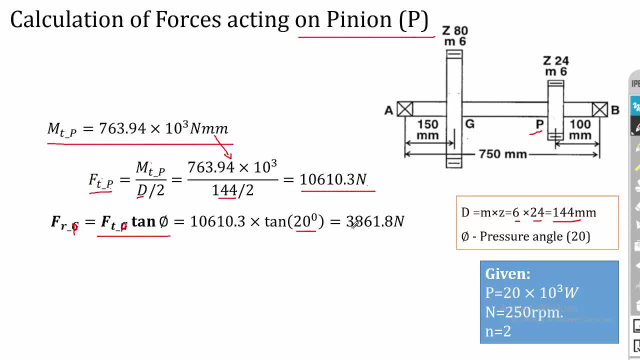 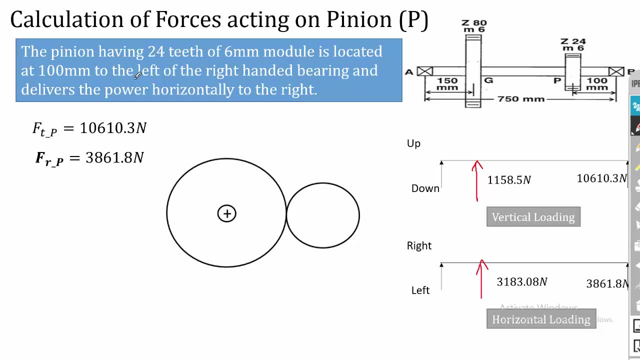 can substitute that and you can calculate. the Frp is equal to 3861.8 Newton. Now we can go for the load drawing. so just read the problem. in the problem it is mentioned that the pinion is located in 100 mm to the right of the right hand bearing and delivers. 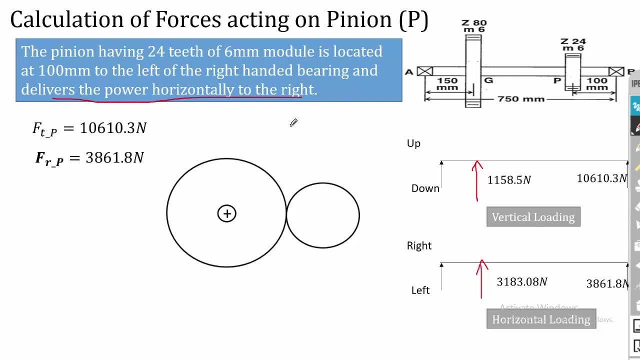 the power horizontally to the right, So it delivers the power, which means the gear is a driving gear. so it's a driving gear, dr. and the mating gear is a driving gear, Dr. I have assumed that the shaft is rotating in counter clockwise direction, so the mating 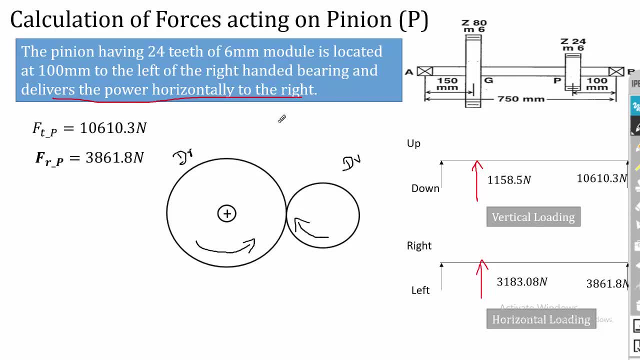 gear will rotate in clockwise direction. So this is very, very important, since the pinion is a driving gear, As I told earlier, always the driving gear will apply the force. so if the driving gear is rotating like this, This driving gear will apply a force. 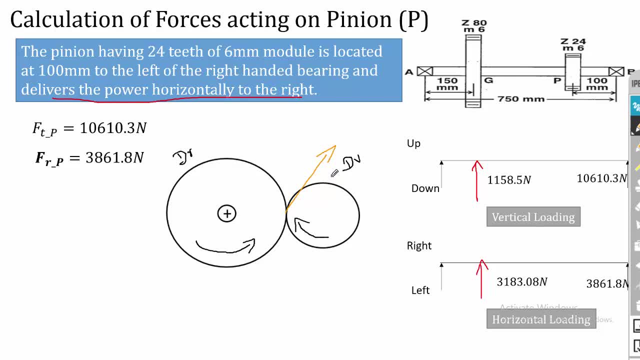 So this force F will act on the driven gear shaft. but we don't want the force acting on the driven gear shaft, so we have to calculate the force acting on the driving gear shaft. So what I am going to do is I am going to draw the reaction force of this force in the 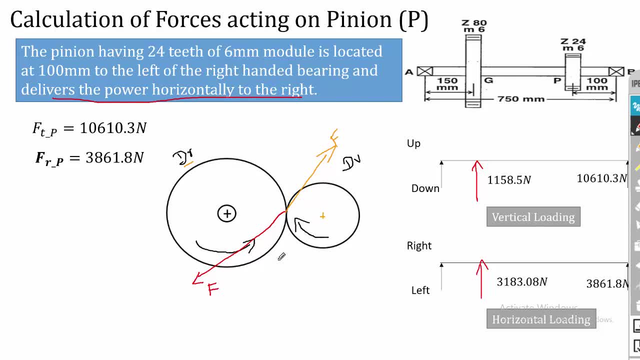 equal and opposite direction with same magnitude. So further I can split this force into two components. One is Ft, a tangential force, because it is acting in the tangential direction and in the radial direction if it is Fr. So if the force is acting away from the gears, then it is tangential. 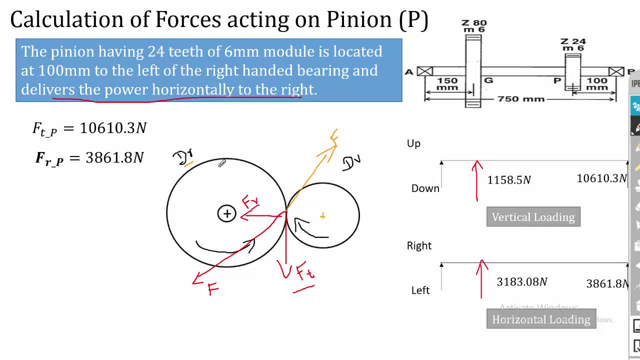 If it is acting towards the axis, then it is radial force. So remember that here it's a driving gear. that's why the driving gear applies the force F, but the applied force is acting on the driven gear, So I have drawn the reaction force. 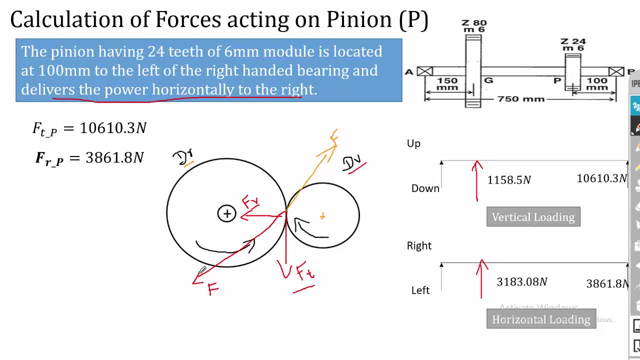 So be clear about it. If the driven gear is fixed in the shaft, then there is no confusion about that. If the driving gear is fixed in the shaft, then we have to draw the reaction force. remember that. So Ftp and Frp we have calculated in the previous slide. 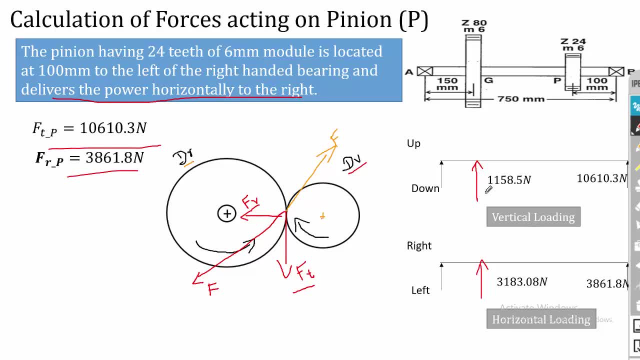 So we can go for the loading drawing. So this is for gear that we have already drawn. Then for pinion, the vertical load. here Ft is the vertical load and it is acting towards downward. So Ft is acting in the downward direction. Then the Fr is a horizontal force and it is acting towards left side. 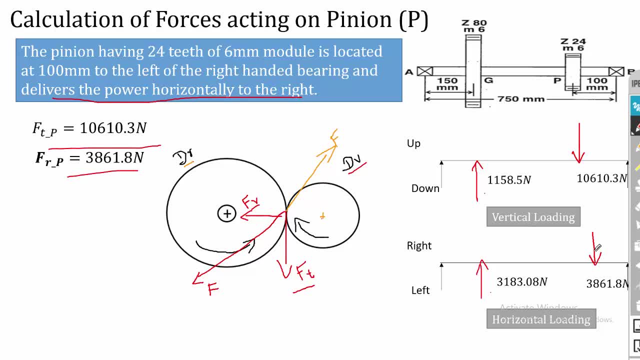 So it is acting towards, from right to left it is going, it is left side. So actually in the problem The weight of the gear or pinion it is not given. So if the weight is given then you have to consider the weight in the vertical direction. 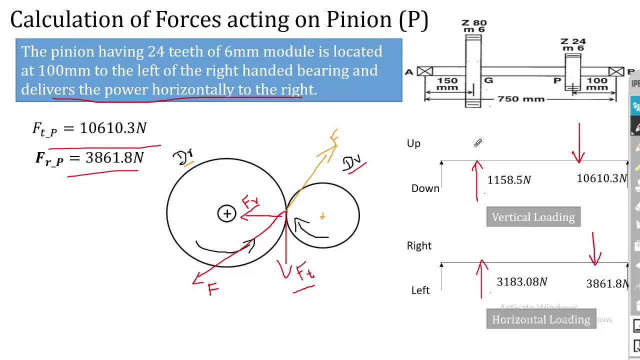 downwards. Remember that the weight will always act in the vertical direction, Since in the problem the weight is not given. I have not considered that If the weight is given then we have to consider in the vertical direction downwards. So this is the force acting on the pinion P. 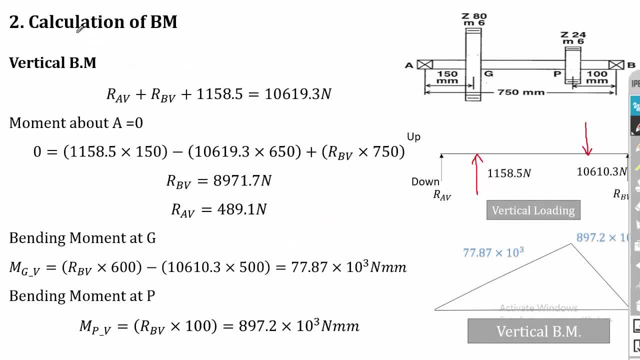 So now we have completed the first step. Then the second step is calculation of bending. Here after the problem is same like the pulley problems. So vertical bending moment. consider the vertical loading. First we have to calculate the reaction force, So the total upward force is equal to total downward force. 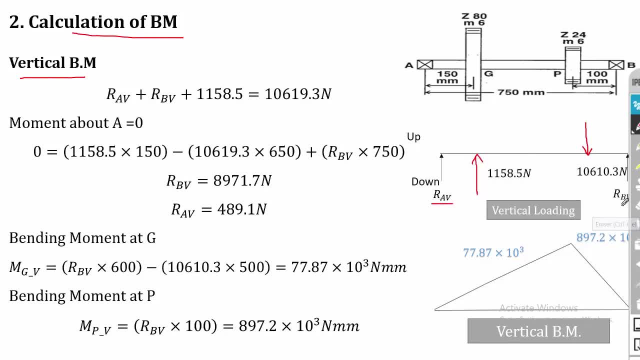 So total upward force is Rav plus Rbv plus 1158.5 is equal to 10600.4.. End, End, End 3 619.3. it is actually okay. fine, then. moment about a is equal to zero. that is moment about. 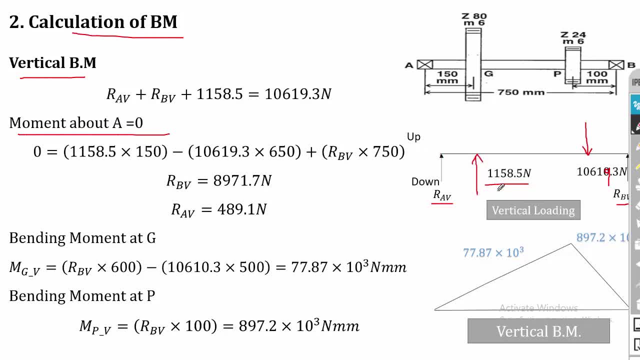 the left extreme point is zero. so the 1158 is acting in the counterclockwise direction, so that is why it is positive. then the 10619 is acting in the clockwise direction. that's why it is negative. then the rbv is acting in the counterclockwise direction, so that's why it is. 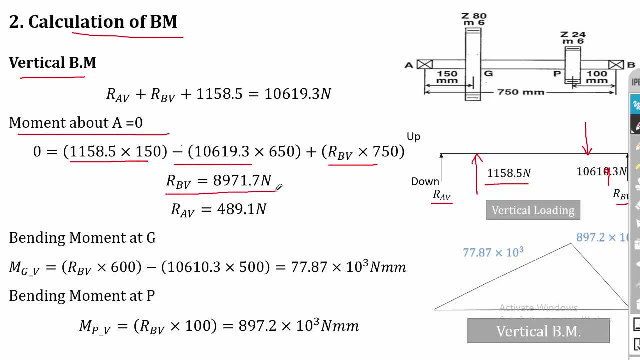 positive. so if you solve this equation finally, you will get: rbv is equal to 8971.7 newton. substitute the rbv value in the first equation and you can calculate the rav value. okay, so now in the drawing we know that the bending moment at a and b is equal to: 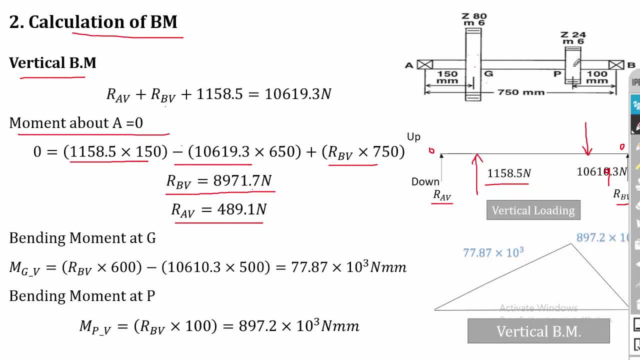 zero. so we have to calculate the bending moment at g and p. so first we'll calculate the bending moment at g, so mg vertical, since it is vertical loading, so it is rbv into 600, since it is counterclockwise, then 1619.3 into 500, that is equal to: 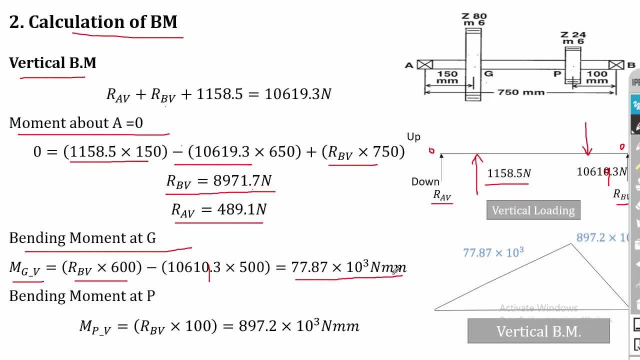 77.87 into 10 power 3 newton mm. then the bending moment at p. we know that how to calculate the bending moment. so you can calculate that mp vertical is 897.2 into 10 power 3 newton mm. okay, so you can draw the vertical bending moment. so after calculating the vertical bending moment, 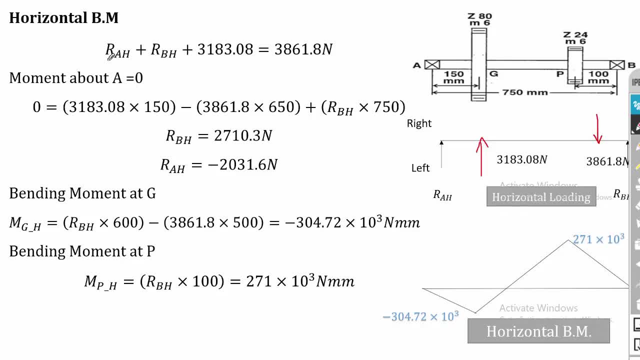 then consider the horizontal loading drawing. so follow the same procedure for horizontal bending movement and you can calculate the bending moment at g and bending moment that p. okay, so the first step is total upward force is equal to total downward force, then the moment about the left extreme point is equal to 0. further, you can calculate the bending. 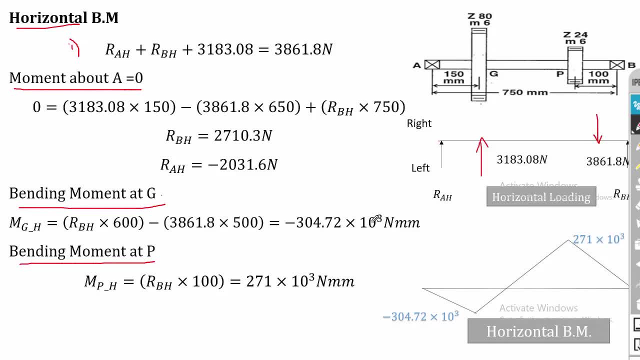 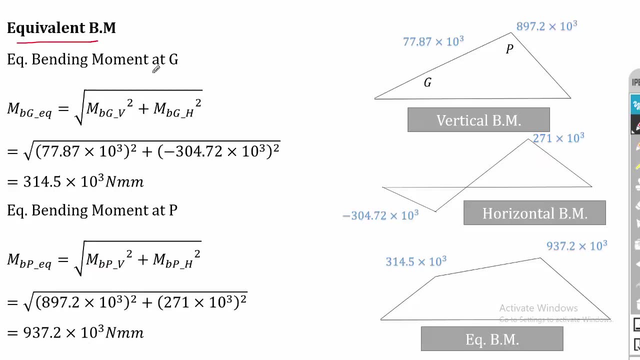 moment that g and p. okay, so remember that at g the bending moment is negative. okay, so this will be your bending moment. bending moment drawing, Don't confuse yourself. So after drawing the horizontal and vertical bending moment, we can draw the equivalent bending moment. So, equivalent bending moment. 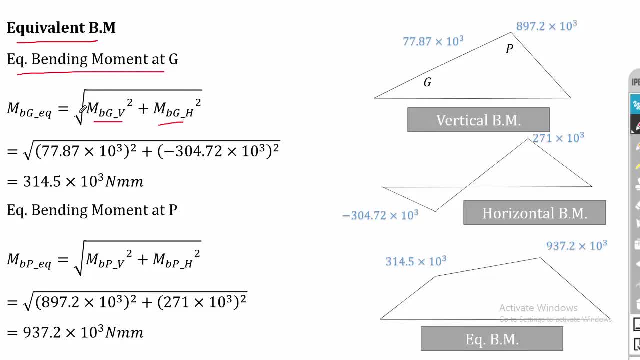 at G is equal to the vertical value square plus horizontal value square. So at G the equivalent bending moment is 314.5 x 10 power 3 Newton mm. Then at P the vertical bending moment is 897 and the horizontal bending moment is 271.. We can calculate the equivalent bending. 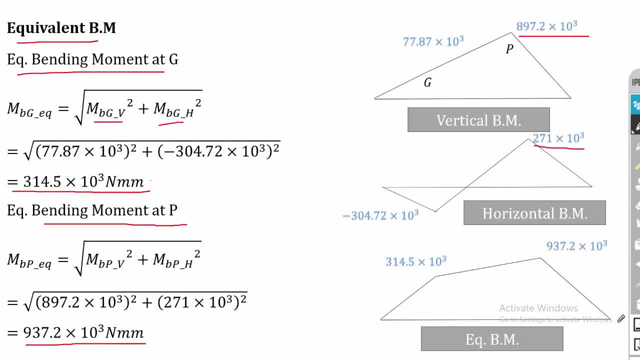 moment and we can draw the equivalent bending moment drawing. So from the equivalent bending moment drawing we can take the maximum bending moment, that is MB. So here in the problem, the MB, the maximum bending moment, occurs at the point P and the magnitude is 937.2. 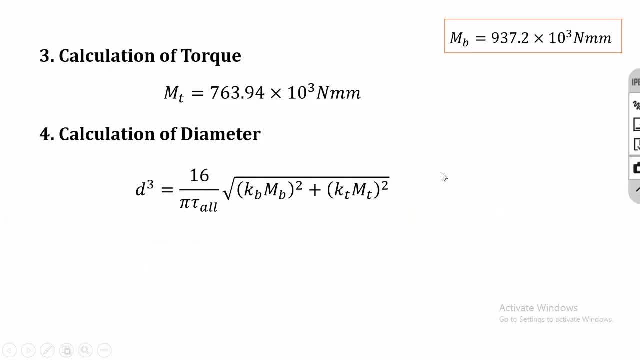 into 10, power 3.. The third step is calculation, Calculation of torque. So torque we have already calculated in the first step. You can take that. Then the last step is calculation of diameter. So since the shaft is subjected to both bending and twisting moment, then it comes under case 3.. We can use this equation. 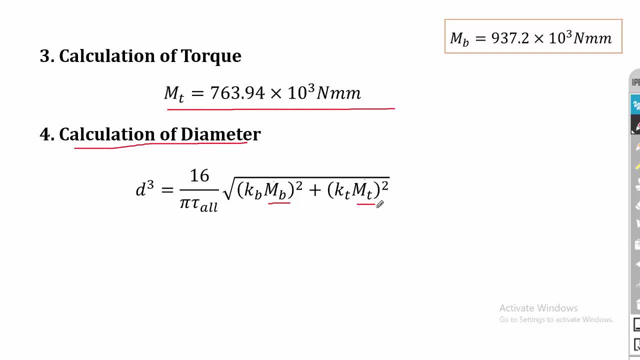 So here MB is the maximum bending moment and MT is the maximum torque. So tau allowable is the allowable shear stress. In the problem the material is not given, So we have to select a suitable material. So what we have to do is we have to select a suitable material. So what we have to do 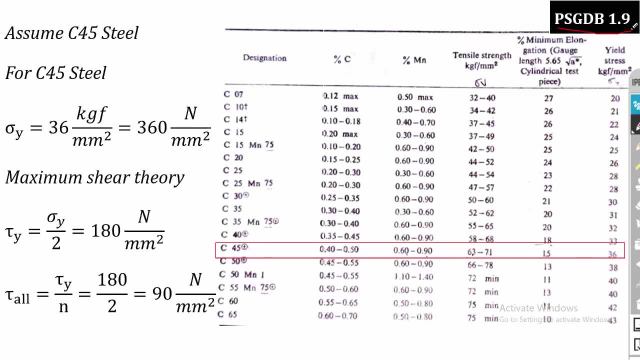 is. I am going to turn page no 1.9 and I am going to select a material of C45 steel And for C45 steel the sigma y value is: you can see that it is 36 kgf per mm square If. 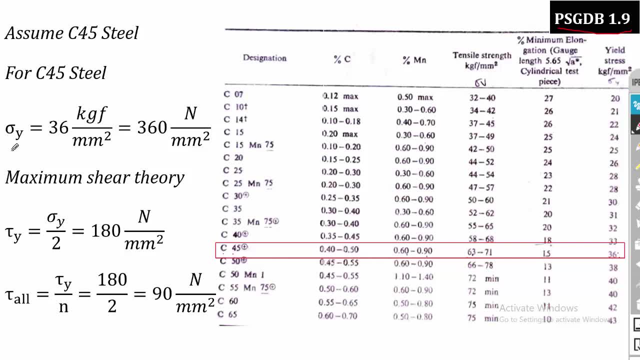 it is 36 kgf per mm square. then sigma y is equal to 360 Newton per mm square. Then sigma: We know that tau y is equal to sigma y by 2, substitute the value of sigma y, you will get tau y is equal to 180 newton. 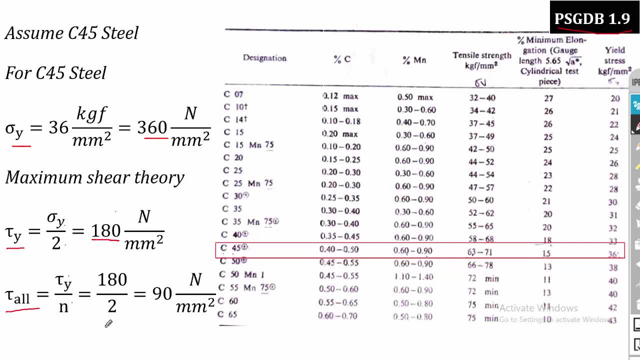 Further, the tau allowable is equal to tau y divided by factor of safety. In the problem the factor of safety value is given as 2, so it is 180 divided by 2, that is equal to 90 newton per mm square. 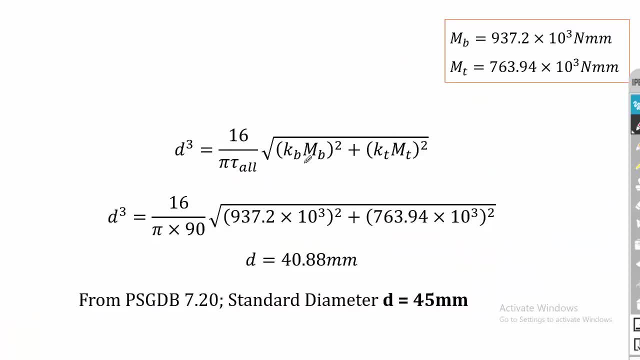 So now we can substitute in the equation, substitute the bending moment mb, the maximum bending moment that we have calculated, then the mt value. So in the problem the kb and kt values are not given. So if it is given then we have to consider that or otherwise we can assume a value of 1 for kb and kt. 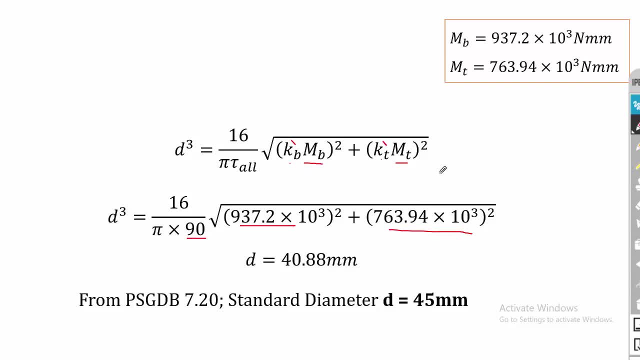 So tau allowable, we have calculated, we can substitute that. So, finally, if you solve this equation, you will get: d is equal to 40.88 mm. So, after calculating the diameter, the next important step is standardizing the diameter, So by using R20.. 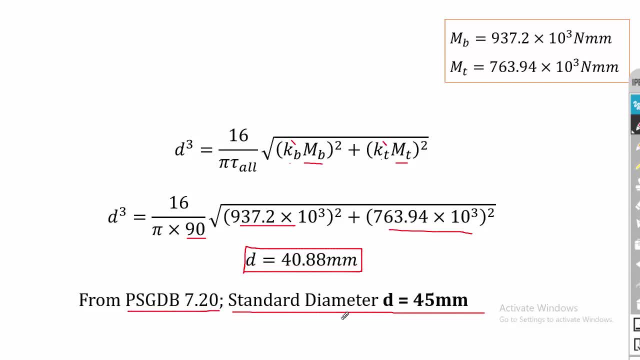 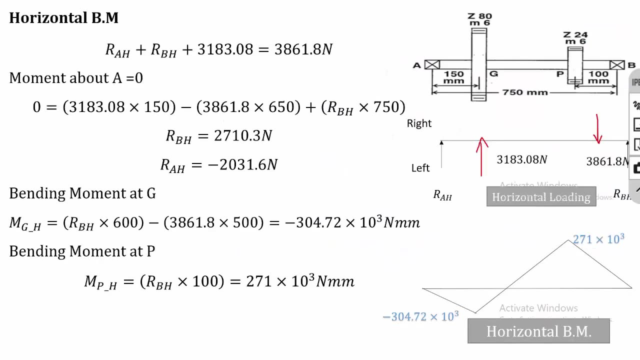 R20 series, in page number 7.20, the standard diameter can be calculated and it is equal to 45 mm. So this is how we have to solve the problems on gears. So the first step is calculation of forces, and remember that first be clear about that, whether your gear is a driving gear or a driven gear. 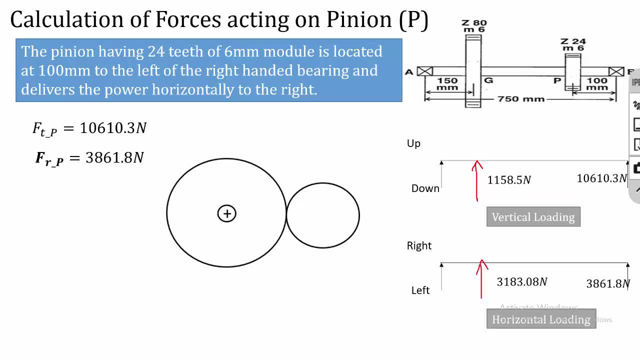 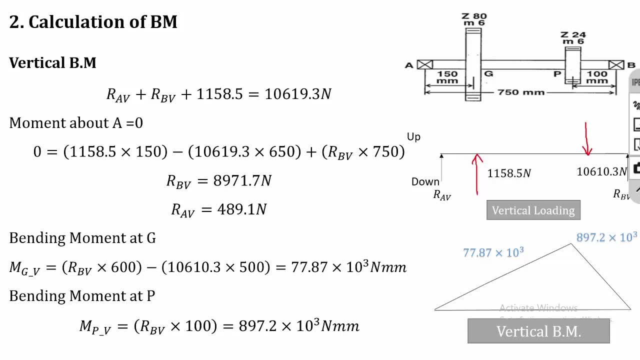 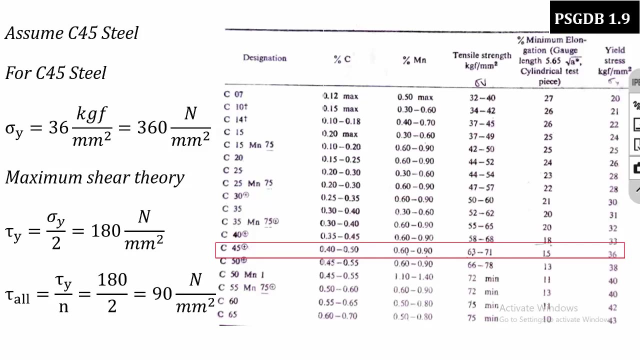 So if it is a driven gear, then directly you can draw the force. If it is a driving gear, then you have to draw the force and from the force you have to take the Reaction force. okay, fine, Then after calculating, after drawing, the force, drawing, then the remaining procedure is same. 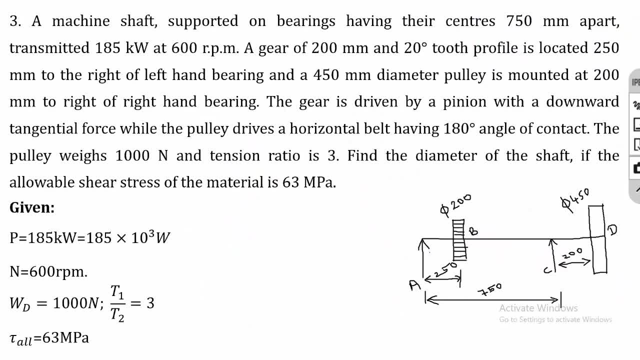 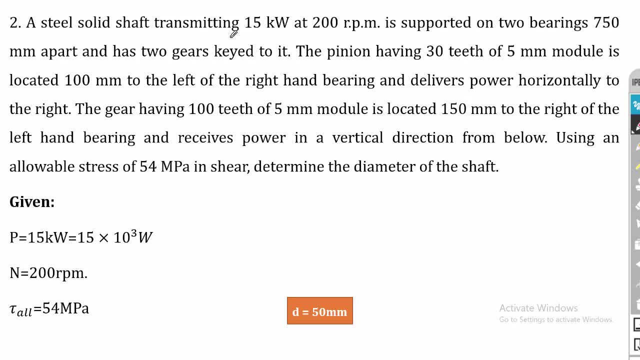 Calculation of bending moment, then selection of torque and calculation of diameter. The tutorial problem: a steel solid shaft transmitting 15 kW at 200 rpm- so the power is given as 15 kW and the speed is 200 rpm- Is supported on two bearings. 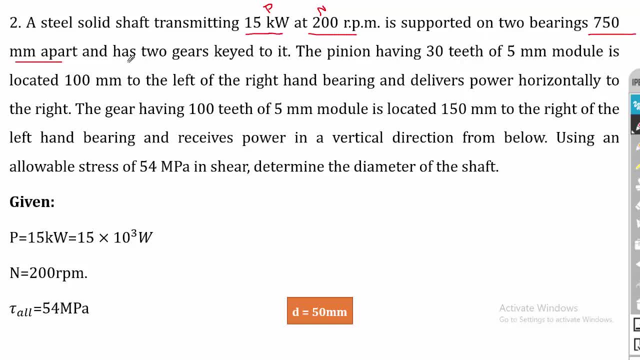 So you can keep this The opinion, having a 30 tissue 5 mm module is located 100 mm to the left of the right hand oser, so you can draw a simple one. It is supported in bearings and the distance is. 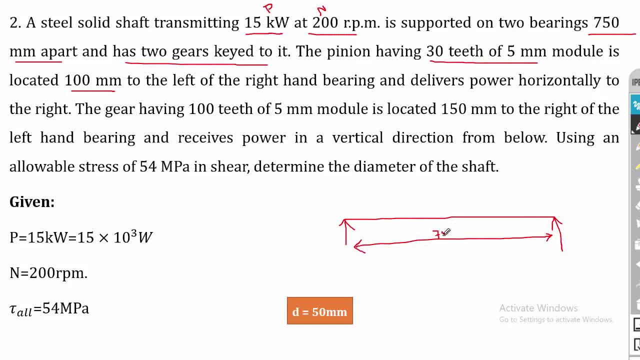 JESSI 750. okay, principles memory. so it's having a pinion at a distance of 100 mm from the left of the right handed bearing And delivers power horizontally to the right. So this pinion delivers power means it's a driving gear. 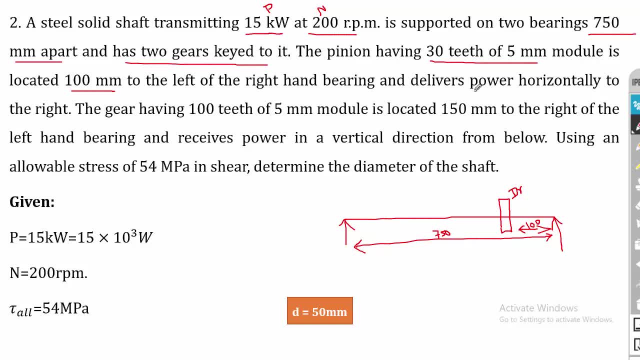 So we have to draw the reaction force, be clear about it. And the next gear is on the horizontal right side. So if you draw the force drawing, then it will be like this: This is your pinion and this is the mating gear. 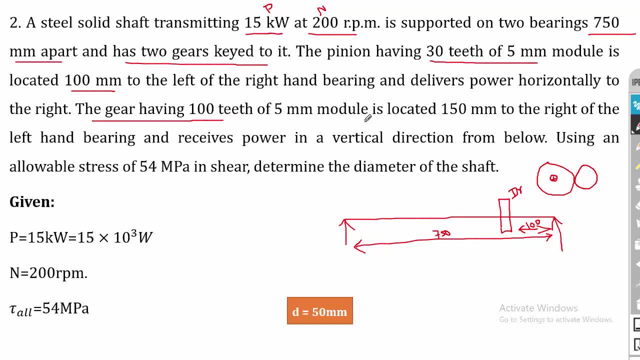 Then the next one. the gear having 100 teeth and 5 mm module is located 150 mm to the right of the left handed bearing. So another gear is located at a distance of 150 mm from the right of the left handed bearing. 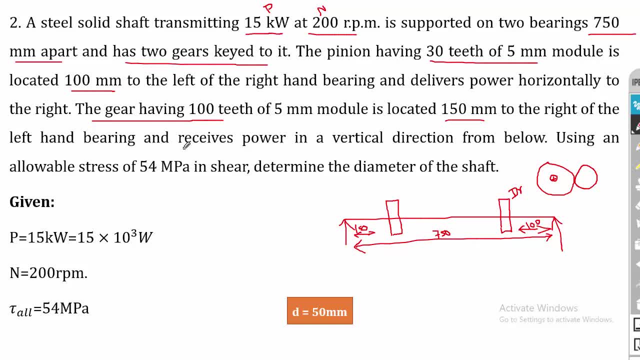 So 150 mm from the left, From the right of the left handed bearing, and receives power in a vertical direction, from below. So it receives the power which means it's a driven gear. So driven gear means you can directly draw the force And it receives power vertically below.